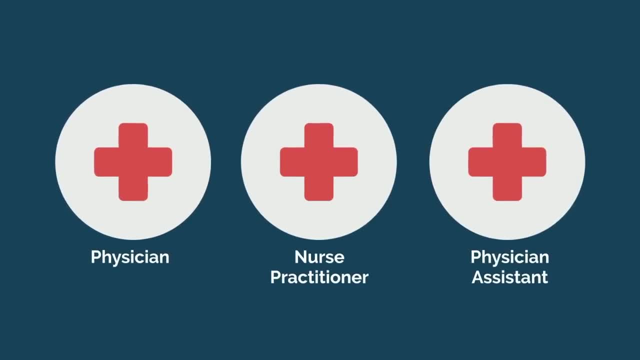 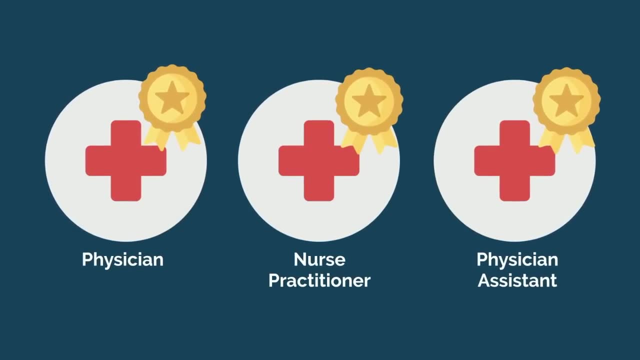 vice versa. Do note that all three are fantastic professions and no single one is better than the other. You simply need to decide what you value most and choose accordingly. This is a big picture overview of the three paths. If you want to dive deeper into any single, 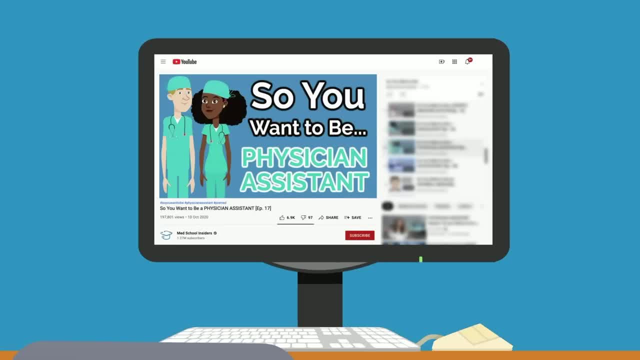 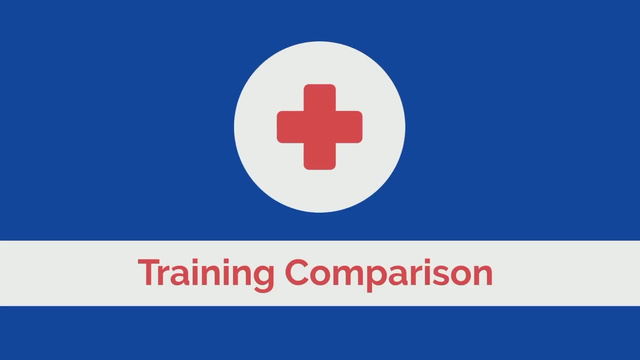 one we have. So You Want To Be episodes for physicians, PAs and NPs Links in the description. Let's start with the different training paths, As this is one of the biggest differentiators and a big reason many choose the mid-level. 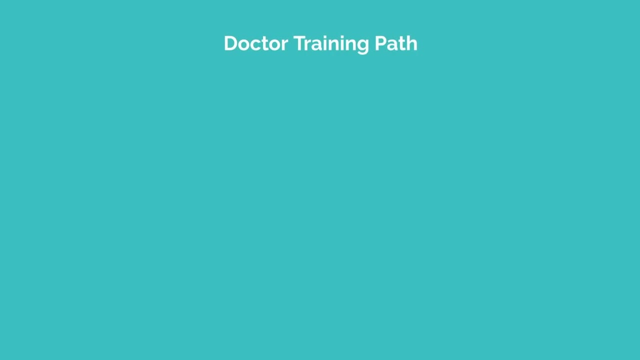 path over the physician path. The doctor training path, whether MD or DO, is the longest by far. After your four pre-med years in college, you'll complete another four years of medical school, followed by three to seven years of residency in your intended specialty If you want to further subspecialize. 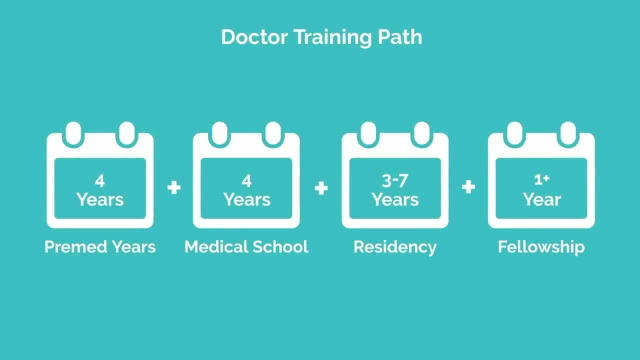 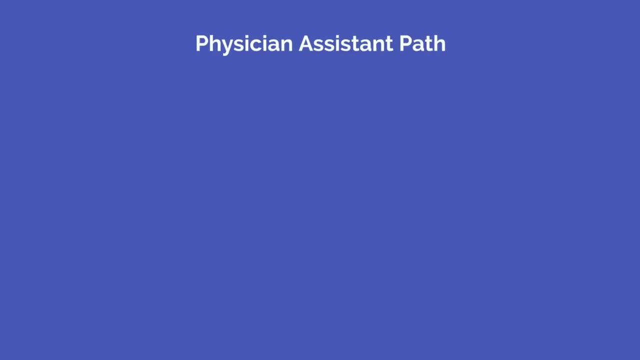 with a fellowship. add one or more years after that. Both mid-level training paths, whether PA or NP, are comparatively much shorter. To become a physician assistant, you'll enter physician assistant school after college, which is two or two and a half years in duration, Whereas in medical school you spend two years. 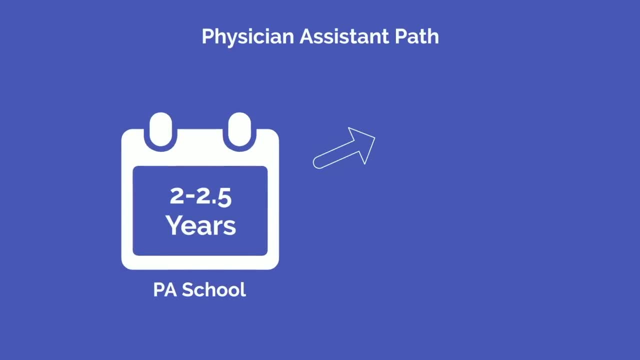 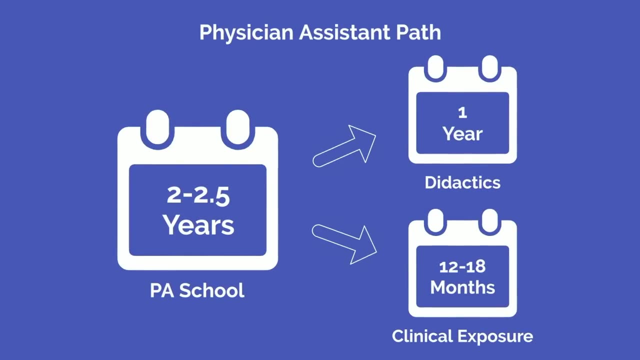 focused primarily on didactics and two years focused primarily on clinic time. in PA school you'll have just one year of didactics and the remaining 12 or 18 months focused on clinical exposure. After that there's no residency and you're free to start practicing as a 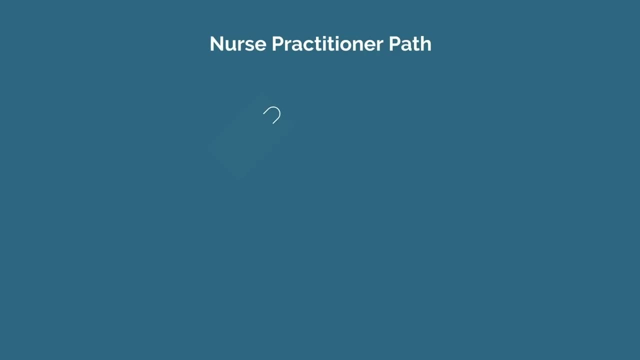 PA immediately. To become a nurse practitioner, you can choose from the following three paths: First, you'll have to be a nurse practitioner. Second, you'll have to be a nurse practitioner. Third, you'll have to be a nurse practitioner. Fourth, you'll have to be a nurse practitioner. 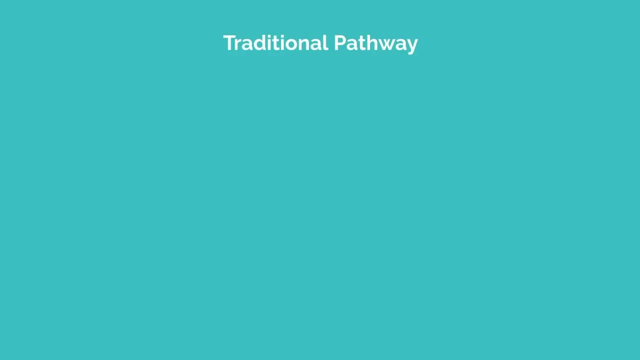 You can choose from two paths: traditional or direct entry. The traditional pathway involves first earning your BSN, ABN or MSN to become an RN, after taking your NCLEX exam. Next, they attend a master's or doctorate program to become an NP If you attend a full-time. 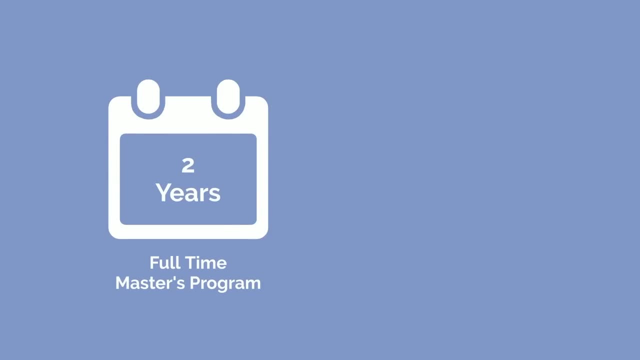 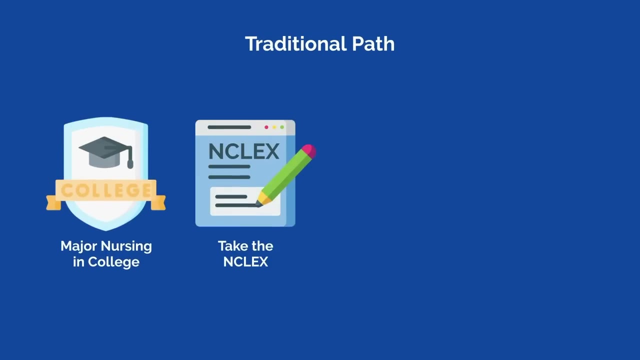 master's program. it will generally take two years, but if you are undergoing a part-time DNP program it can take up to five. If you were to major nursing in college and take your NCLEX, you could become an RN soon after graduation. And because you're a nurse practitioner, you can choose from two paths. 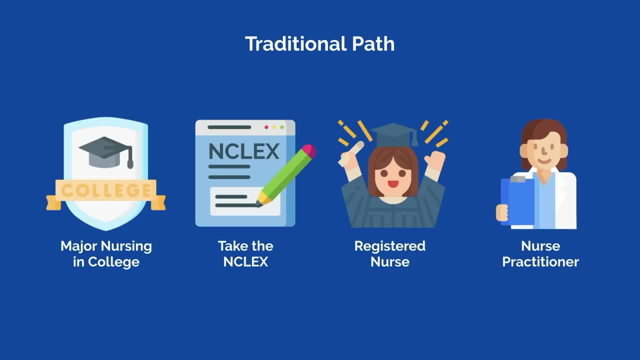 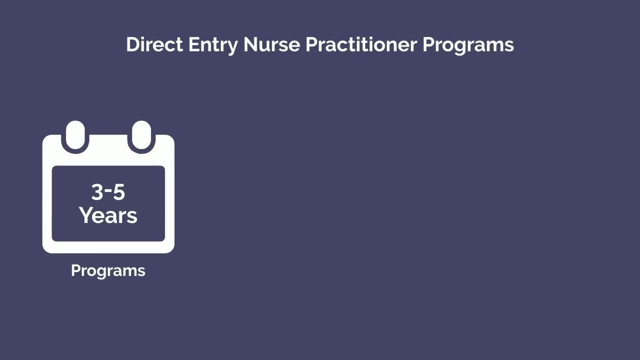 Traditional or direct entry. The traditional pathway involves first earning your BSN, ABN or MSN to become a fully trained NP just two years later. The second pathway, or direct entry, nurse practitioner programs are for those who earned a bachelor's degree in something else. These are three to five year programs where you 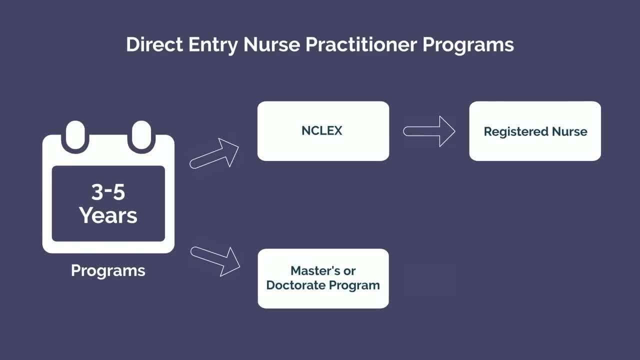 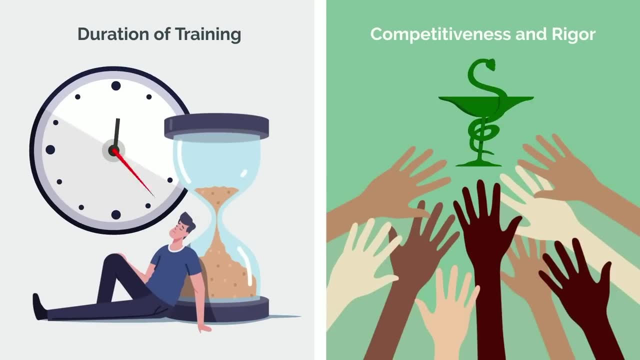 will take both the NCLEX to earn your RN, but also complete a master's or doctorate program to become an NP. It's not just the duration of training but also the competitiveness and rigor of each path. Getting into medical school is by far the most competitive of the 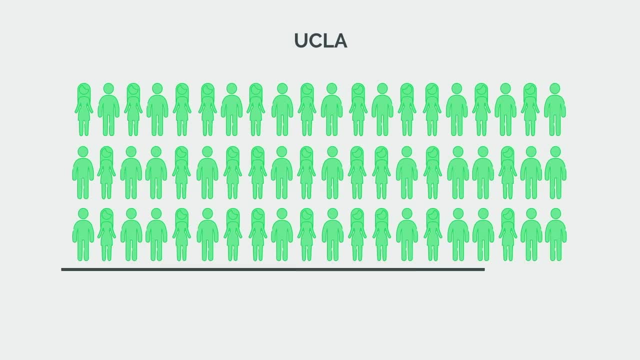 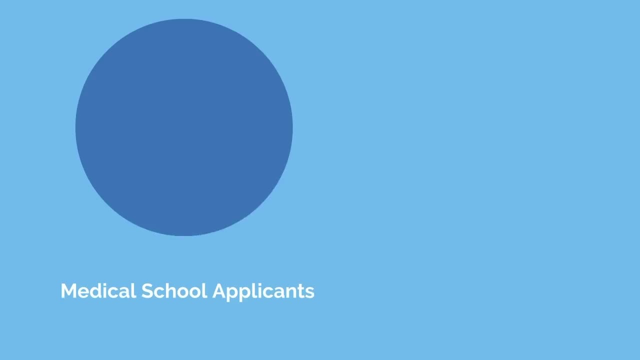 three. At some schools, like at UCLA when I was there, over 80% of premeds on the first day of college are no longer premeds by graduation time And of those who do ultimately apply to medical school, only 40% get accepted. The average: 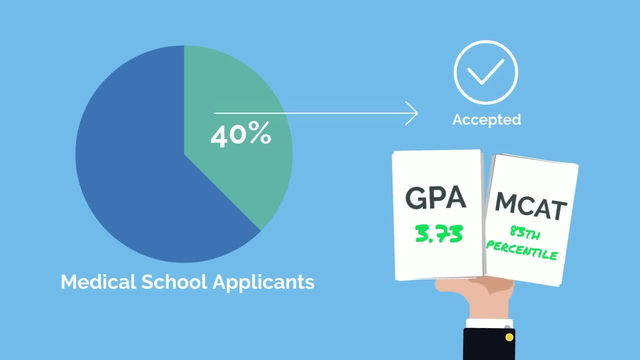 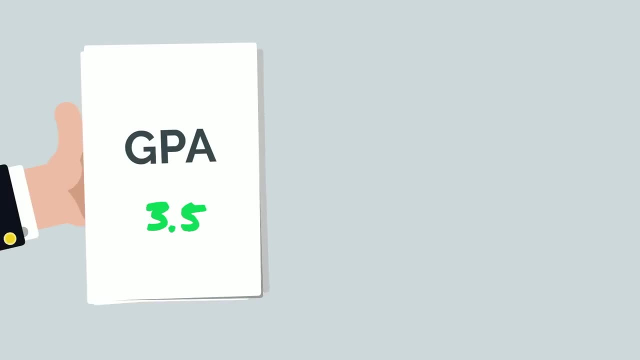 matriculant stats are 83rd percentile on the MCAT and a 3.73 GPA. After medical school, PA school is next in the order of competitiveness. The average GPA for accepted PA students is 3.5, and they average around the 40th to 50th percentile. 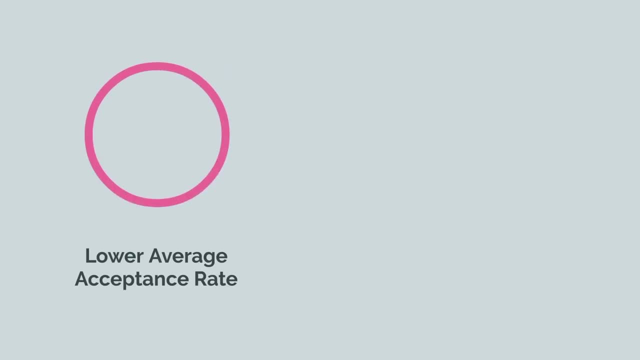 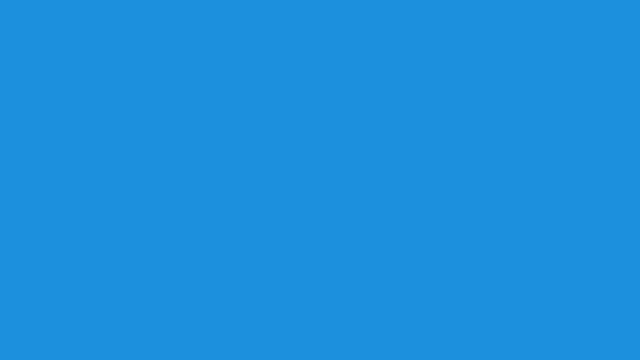 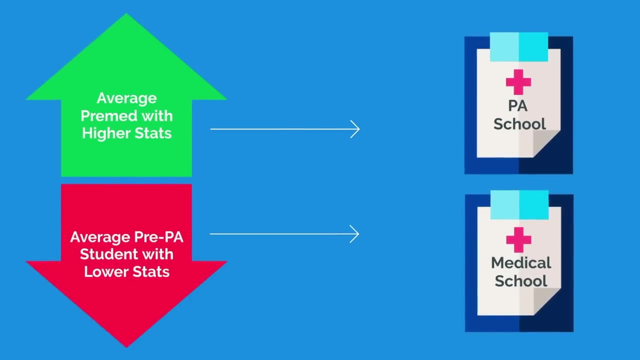 on the GRE, Note that they do have a lower average acceptance rate at 33% of all applicants, and this sometimes confuses students into thinking PA school is more competitive When you consider the outcome if the average premed with higher stats applied to PA school or the average pre-PA student with lower stats applied to. 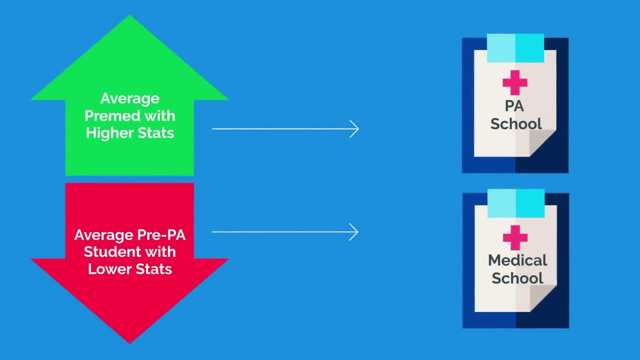 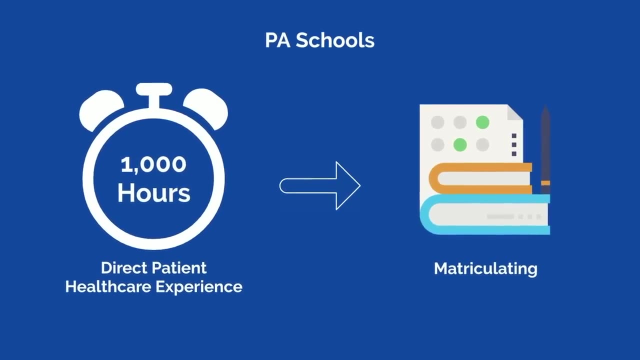 medical school. it generally clarifies any confusion. Do note that many PA schools also require over 1,000 hours of direct patient healthcare experience prior to matriculating. This does not make it any more competitive, but you will need to spend considerable time. 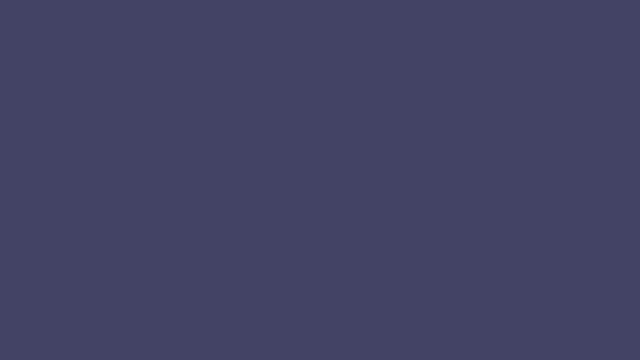 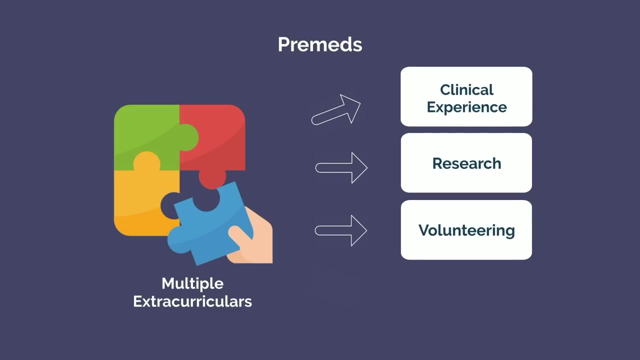 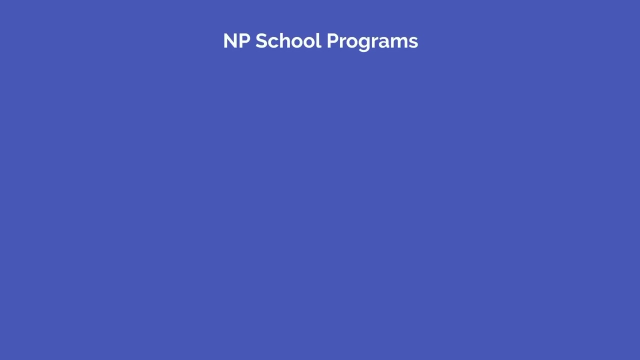 on this. While premeds don't need 1,000 hours of direct patient experience, they do need to put in several hundreds of hours across multiple extracurriculars, including clinical experience, research, volunteering, leadership and others. NP school is the least competitive of the three and it has the loosest requirements. 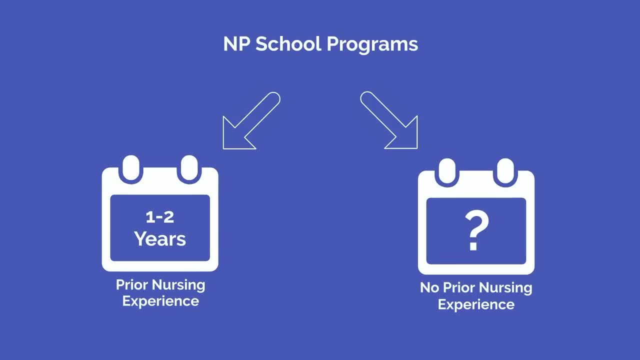 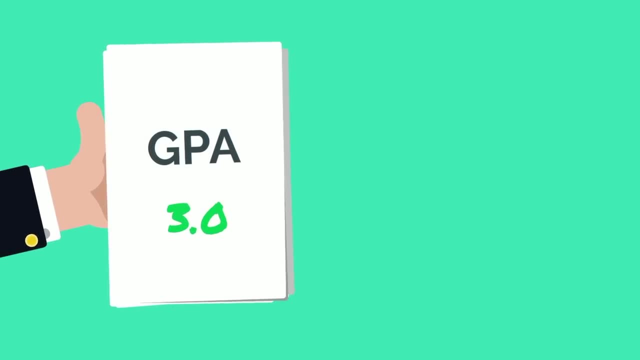 Some programs require 1-2 years of prior nursing experience, while others don't require any. GPA isn't highlighted as a primary factor, with most GPA cutoffs around 3.0, but this isn't a hard rule. Tennessee State University, for example, is reported to generally accept applicants. 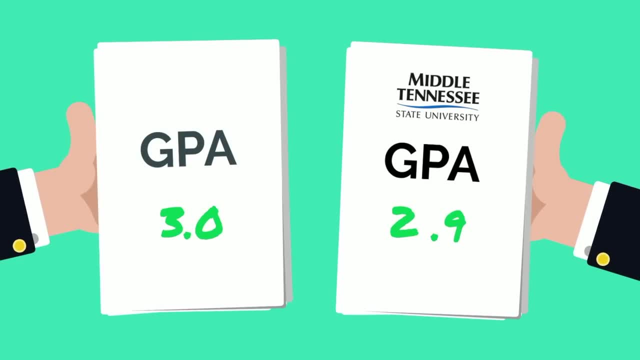 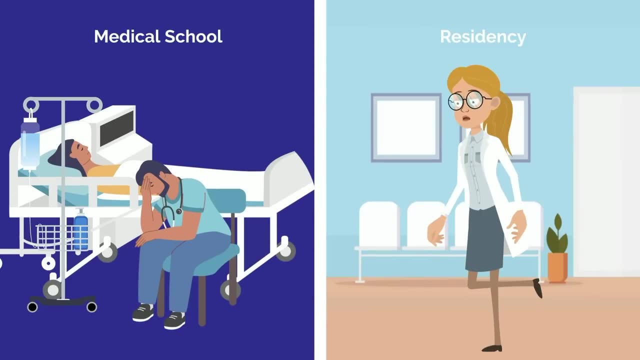 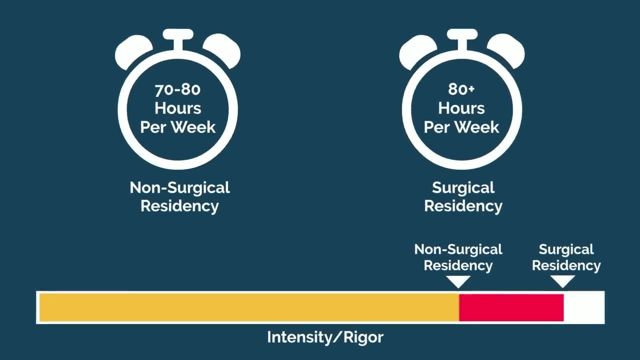 with a GPA of 2.9 or greater. When it comes to rigor, your clinical years in medical school and your residency years will be extremely trying. The norm is to be working 70 to 80 hours per week, but expect over 80 hours in most surgical specialties. With the PA and NP training paths, you won't. 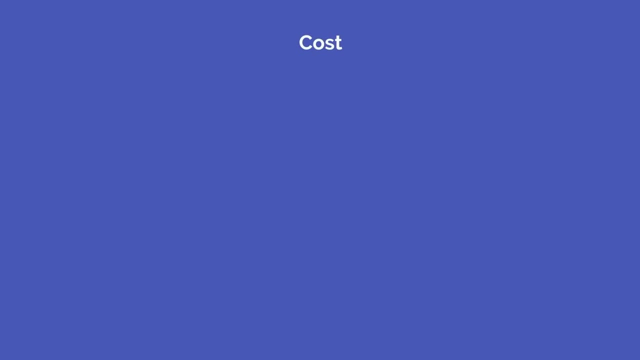 be expected to put in such long hours or for so many years. In terms of cost, medical school is the most expensive, followed by PA school, followed by NP school. The average annual tuition for medical school is $40,000 to $60,000, and graduates have an average debt burden. 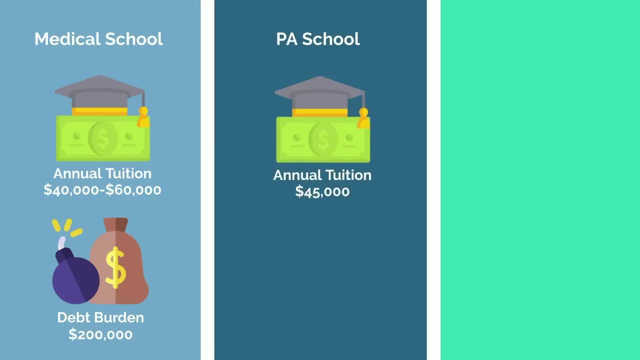 close to $200,000.. The average annual tuition for PA school is about $45,000, with average graduating debt burden approximately $110,000.. NP schools average between $18,000 to $32,000 per year, with the average graduating debt burden between $40,000 and $60,000, depending. 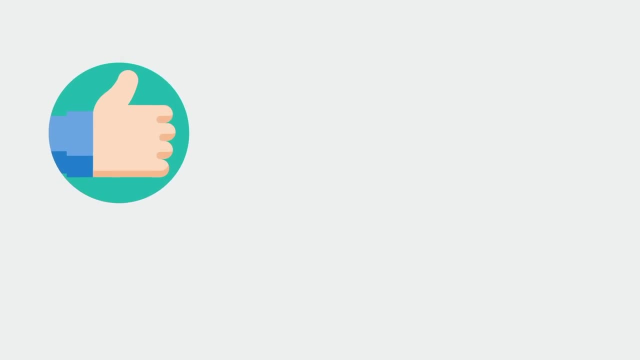 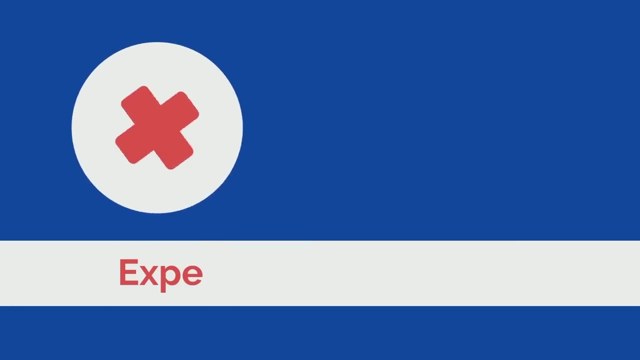 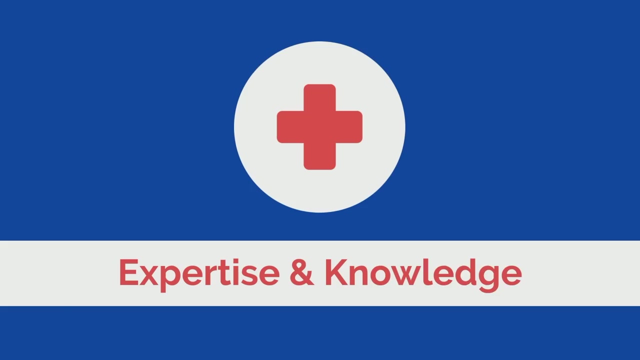 on the source. If you're finding the video helpful, let me know with a thumbs up and consider gently tapping the subscribe button and notification bell. with surgical precision, Considering the training paths, it's natural to assume that physicians have the deepest knowledge and expertise when it comes to the body and how to treat its various ailments. 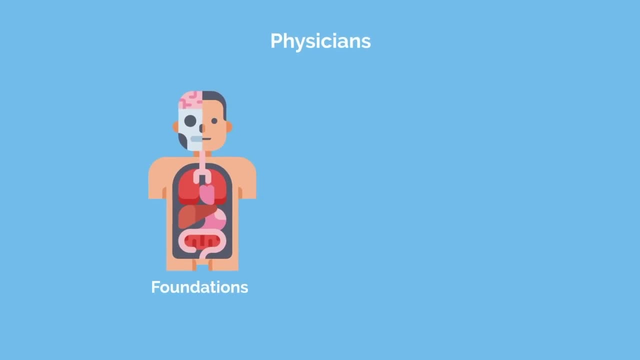 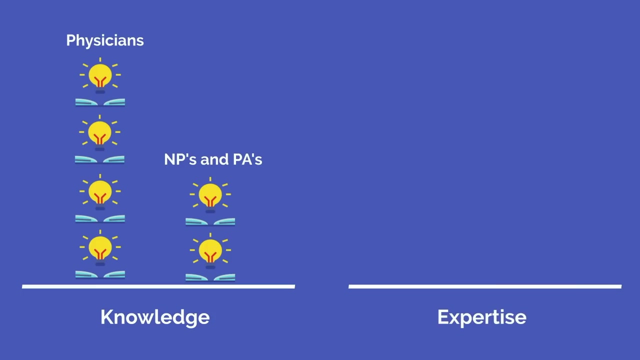 If you assumed that, then you would be correct. Not only do physicians spend the most time focusing on the foundations, but they also spend several years focusing on their specific specialty. in residency, Levels is substantial but, as the name describes, is less than that of physicians, NPs and PAs. 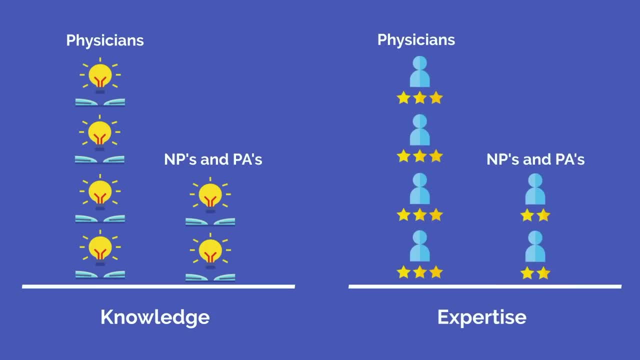 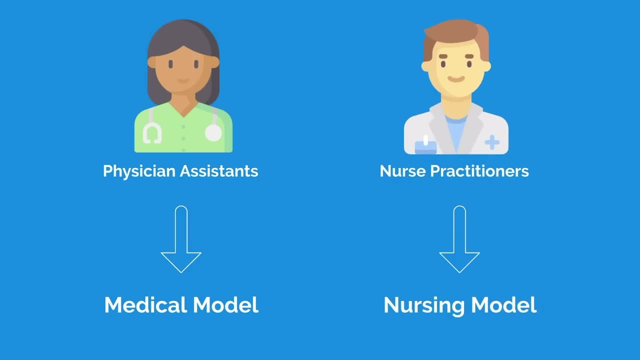 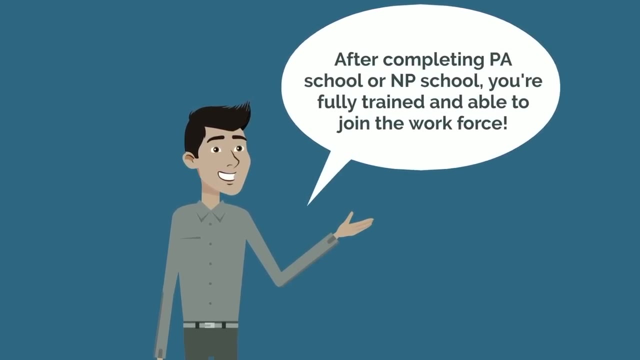 spend far less time in training than physicians and therefore don't have the same depth of expertise. Physician assistants follow the medical model similar to physicians, while nurse practitioners follow the nursing model. But note that after completing PA school or NP school, you're fully trained and able to join the workforce without any required. 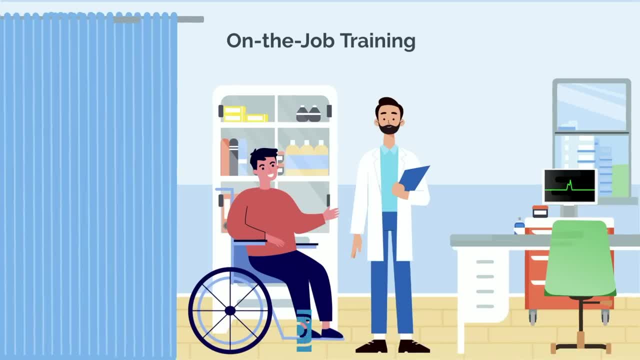 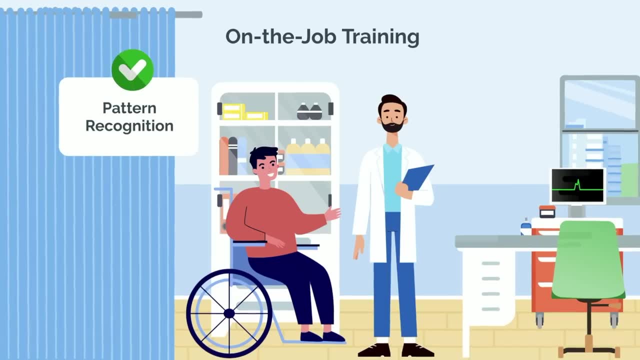 residency for specialty training. PAs and NPs get a great deal of their specialty training on the job after joining a practice. While this is very useful in getting up to speed quickly with pattern recognition for common presenting concerns, you won't be well equipped. 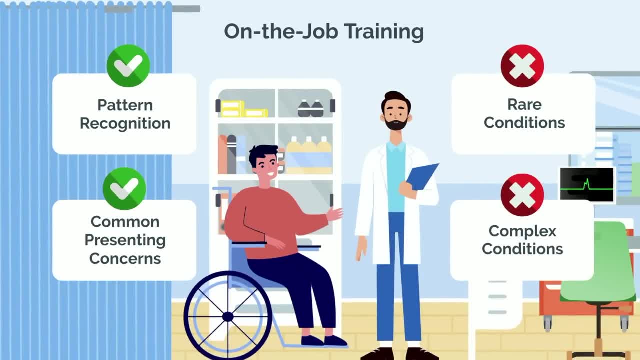 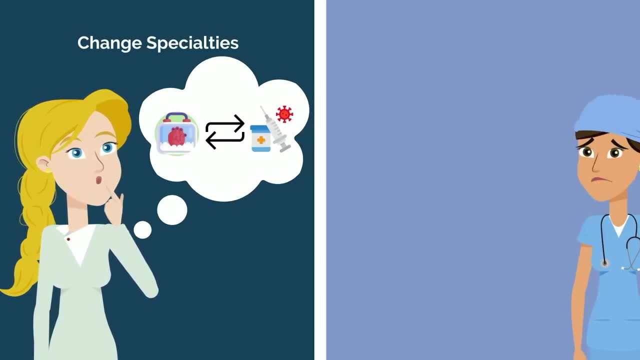 to identify and manage rare or complex conditions. Given the on-the-job training, it's also much easier to change specialties later in your career if you get bored of one or want a change of pace. That's not feasible to do so for physicians who have to reapply. 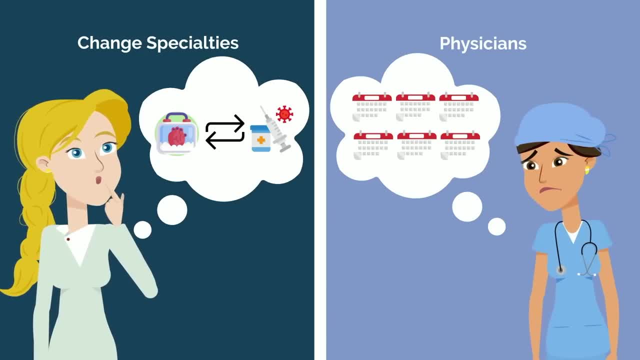 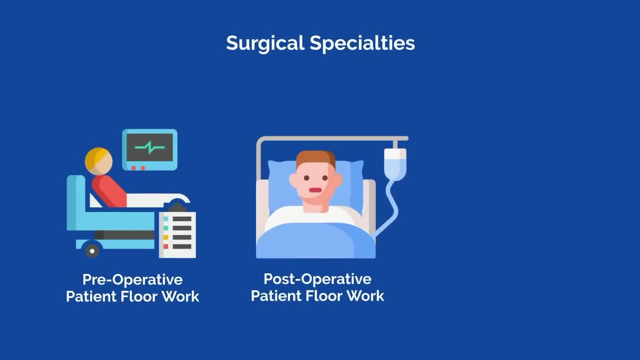 to residency and complete another three to seven years of structured training. PAs are considered to have the most fundamental expertise in the field of physical therapy and the most flexibility, and are sometimes found in surgical specialties either handling pre- or post-operative patient floor work or assisting in the operating room. NPs have flexibility. 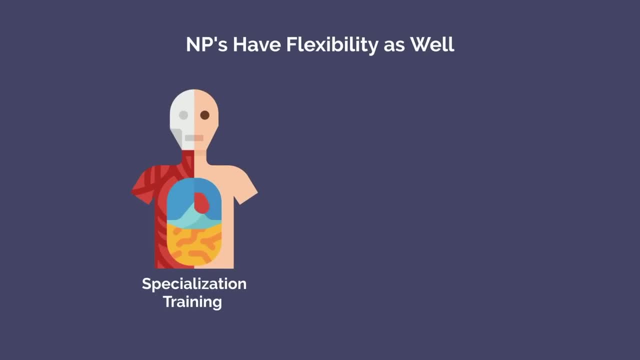 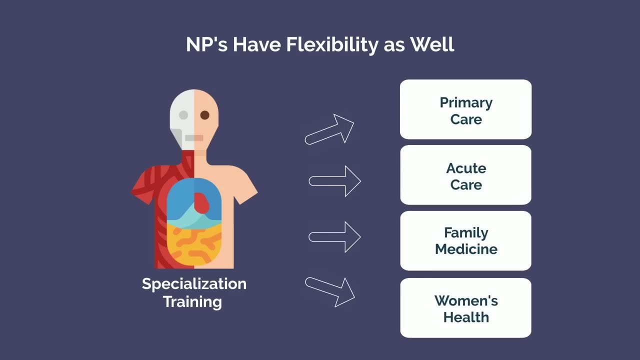 as well, but you'll need to be intentional with which program you attend, as each program trains you toward a specialization, such as primary care, acute care, family, women's health and so on. If you are interested in surgery, note that only surgeons with an MD 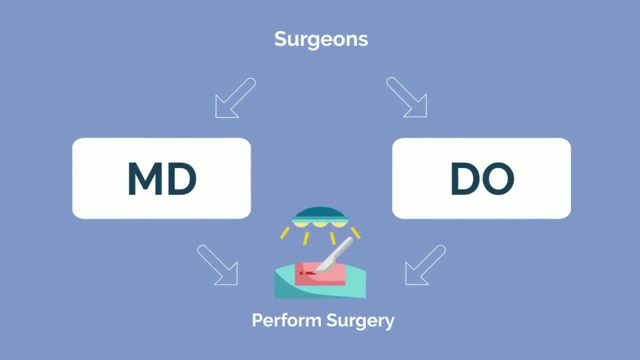 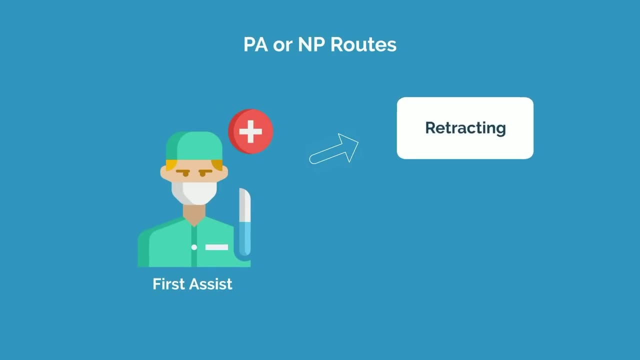 or DO are qualified and have the sufficient knowledge and expertise to perform surgery With the PA or NP routes. the most you'll be able to do in the OR is be first assist, helping the surgeon by retracting, suctioning, suturing and the like. That's the level. 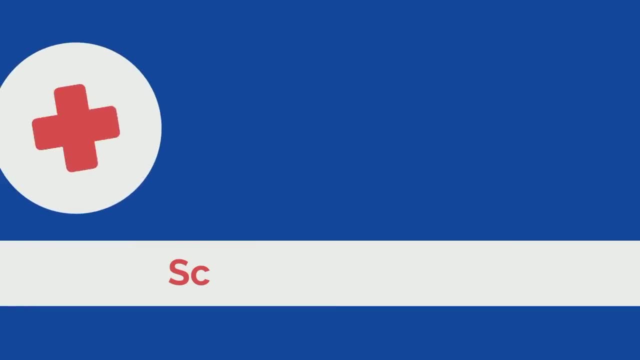 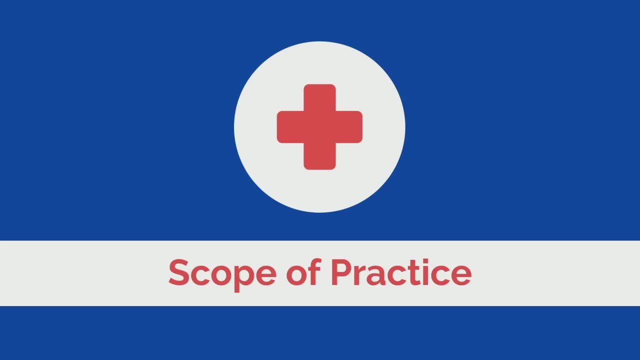 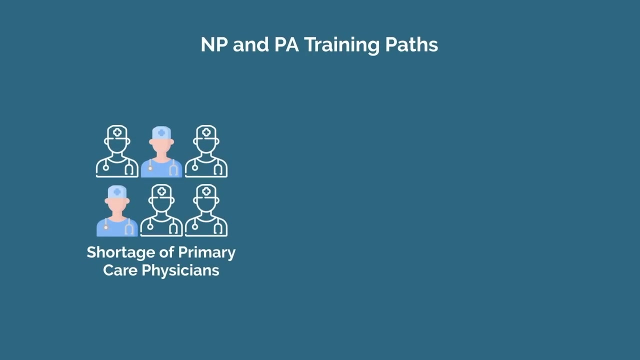 of responsibility of a medical student or junior resident, which brings us to the hotly debated topic of scope of practice. Scope of practice refers to what each type of professional is expected and allowed to do. Historically, the NP and PA training paths were created to address a shortage of primary care physicians and were to serve as an adjunct to physicians In the past. this has been the case for a number of patients, but it's not the case for all of them. In the past, there has been a shortage of primary care physicians and were to serve as an adjunct to. 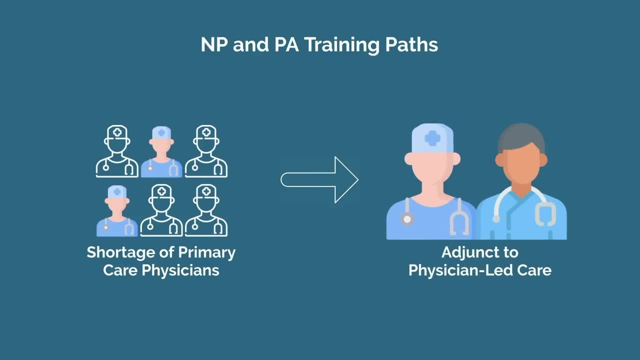 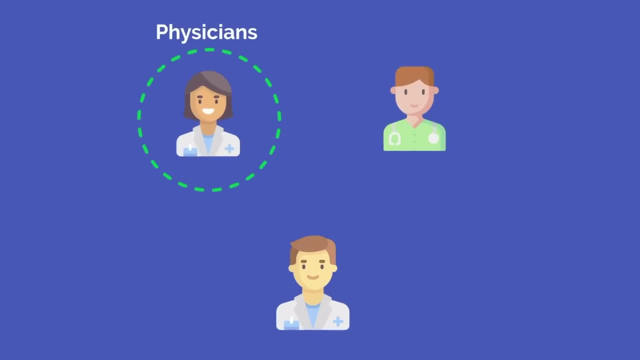 physician-led care, not as a replacement. In this model, NPs, PAs and physicians all work together in harmony in service to the patient, Since physicians have the most robust knowledge and training. mid-levels were generally working alongside physicians and would easily 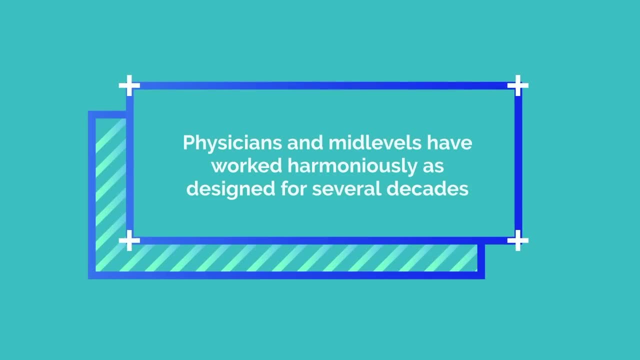 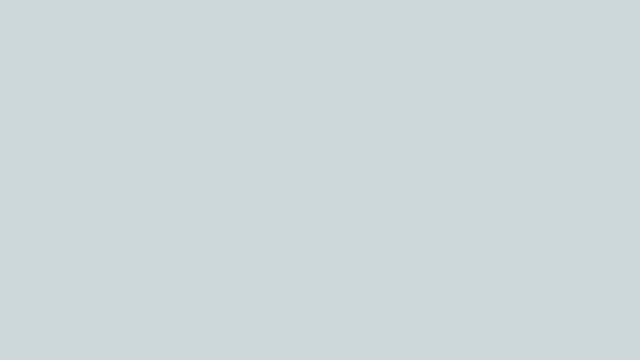 be able to ask for assistance on more complex or rare presentations. Physicians and mid-levels have worked harmoniously, as designed, for several decades. However, in recent years, there's been a growing power struggle between physicians and mid-levels over scope of practice. 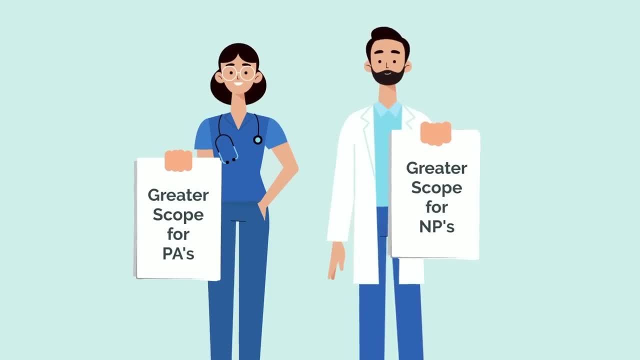 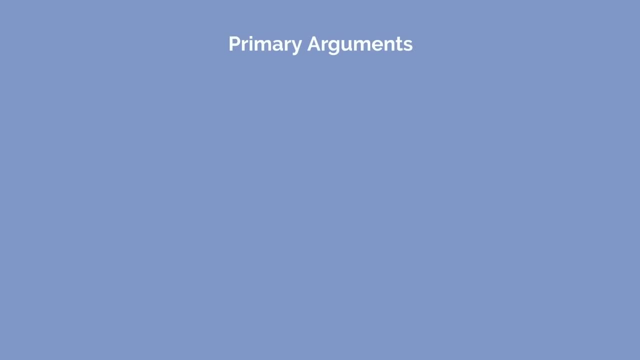 On one hand, NPs and PAs are lobbying for greater scope, meaning they want to do more things physicians traditionally do, such as independent practice. The primary arguments are two-fold. First, we have a shortage of primary care physicians and mid-levels can. 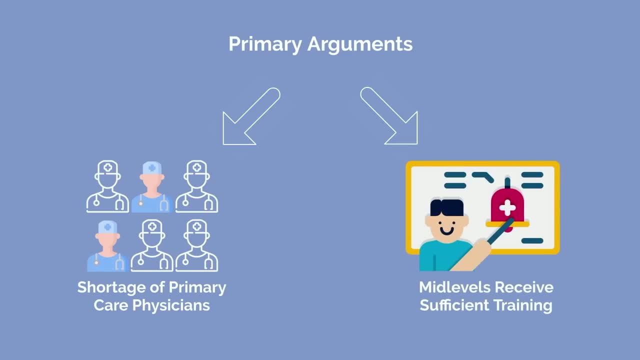 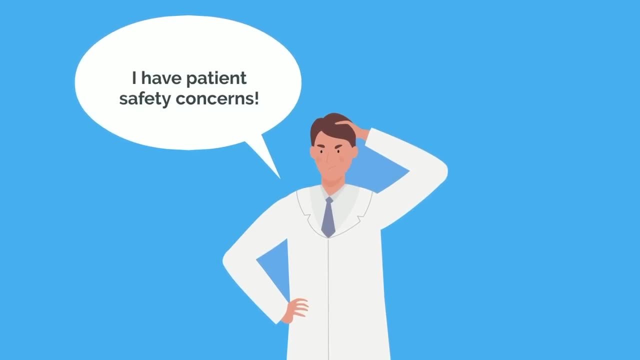 help alleviate that. And second, they argue that mid-levels receive sufficient training to practice independently and safely. On the other hand, physicians are pushing back, primarily focused on patient safety concerns. After all, NPs and PAs receive far less training. 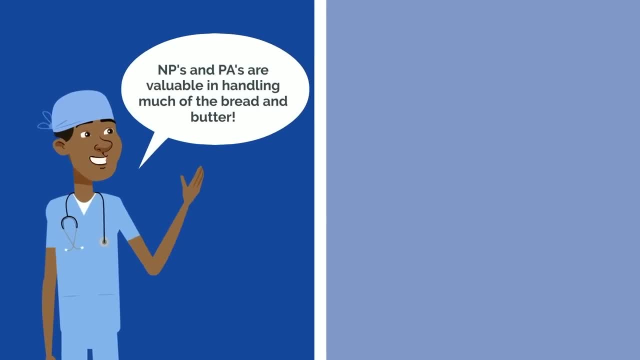 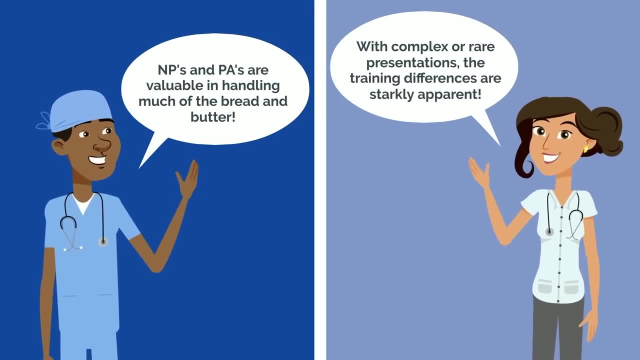 compared to mid-levels My physician mentors and colleagues have shared. they find the NPs and PAs in their practice are valuable in handling much of the bread and butter, meaning the most common and simple cases. However, when it comes to a complex or rare presentation, 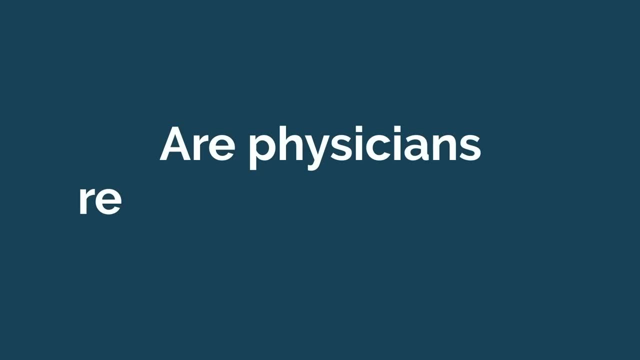 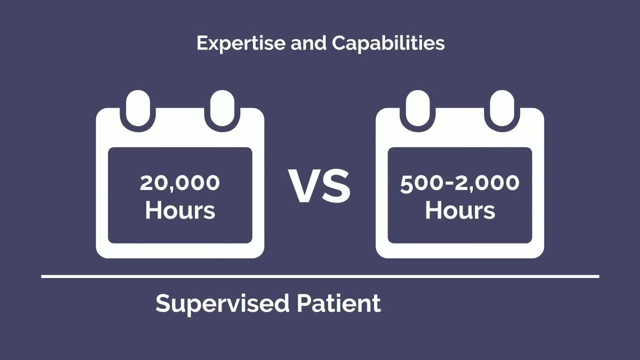 the training differences are starkly contrasted. But are physicians really more qualified? Comparing the expertise and capabilities of someone who receives over 20,000 hours of supervised patient contact compared to just 500 to 2,000 seems like a no-brainer. It would seem obvious that they are more qualified. 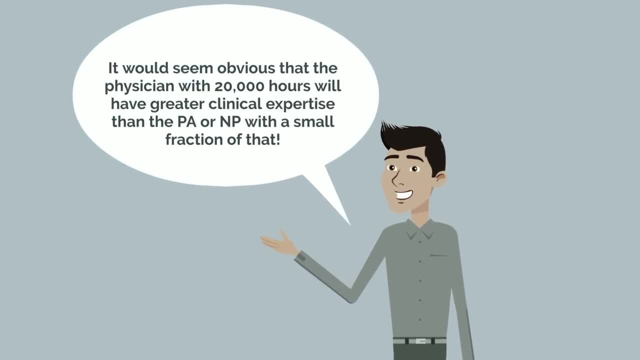 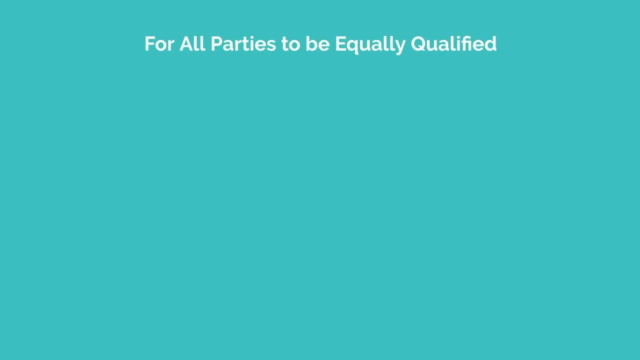 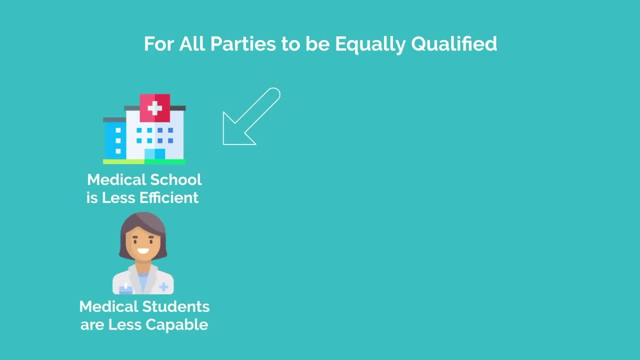 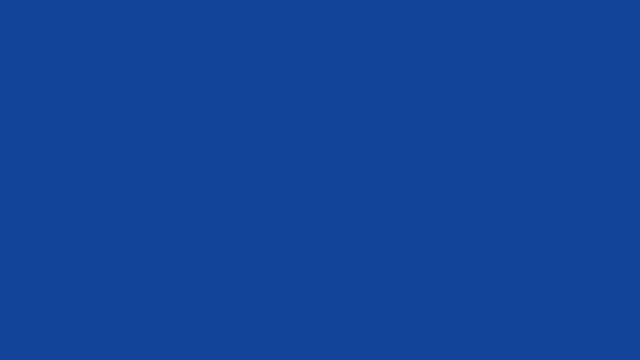 medical school is massively less efficient and medical students massively less intelligent or capable, or if mid-level training paths are massively more efficient and their students massively more intelligent or capable. Scope of practice creep is very, very important, After all, if you're able to do more and practice more independently, similar to a 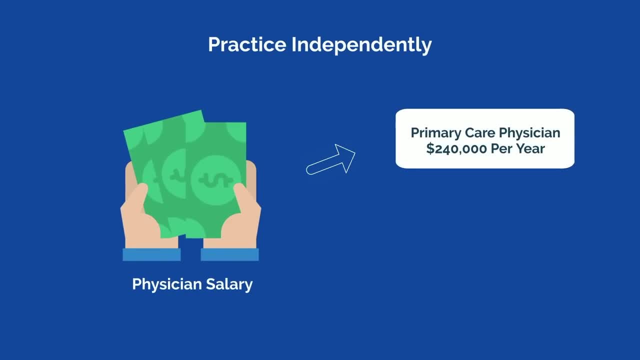 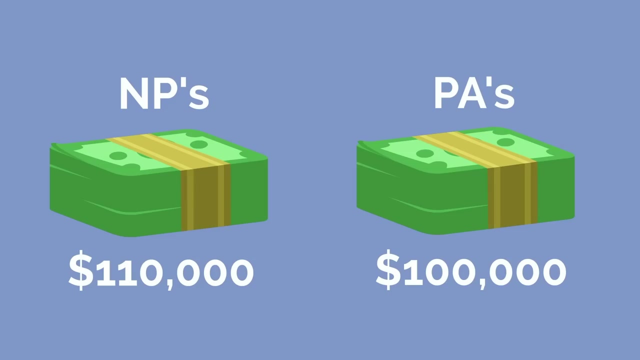 physician, then you can make closer to a physician's salary. The average primary care physician makes $240,000 per year and the average specialist physician makes $340,000.. In comparison, NP's average approximately $110,000 per year and PA's average approximately $100,000. 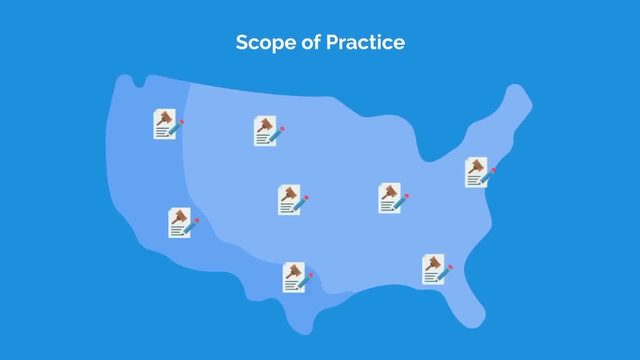 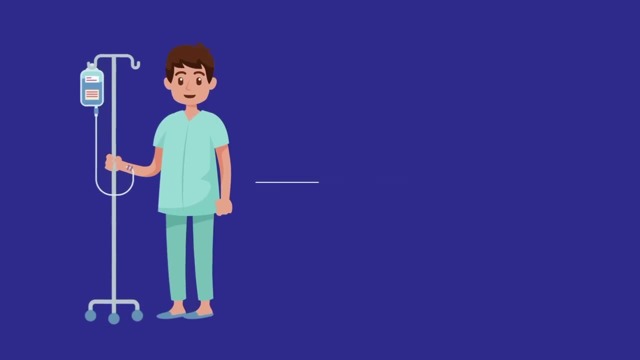 Note that laws governing the scope of practice for each type of healthcare professional vary from state to state, which adds further complexity to the situation. The reason this is important and you should care is because of patient safety, If you or anyone you care about will. 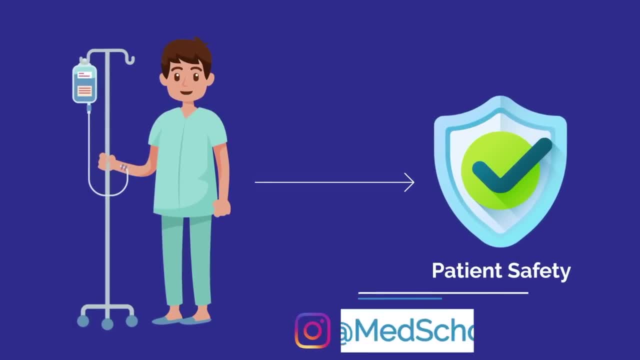 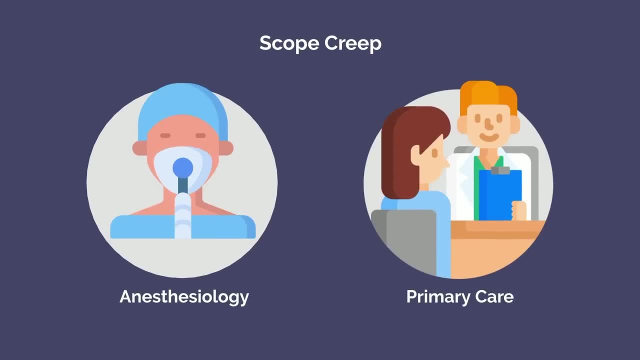 ever receive any medical care, then this is deeply relevant to you. The fields that are currently most significantly affected by scope creep include anesthesiology and primary care, but go on Reddit or MedTwitter and you'll see other specialties cropping up. Ultimately, 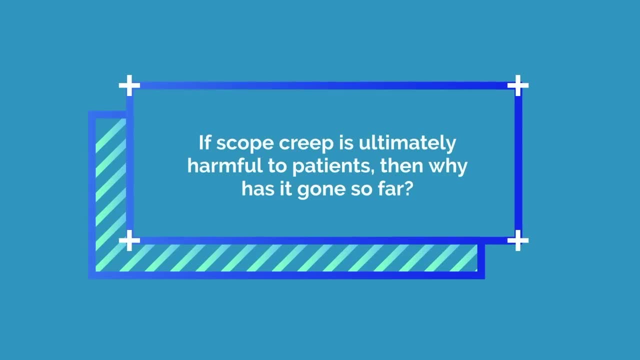 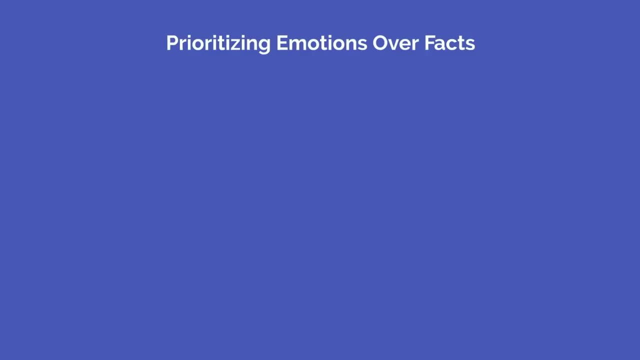 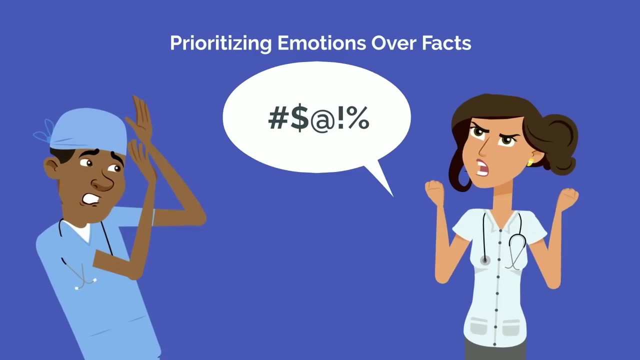 the surgical specialties are the safest from scope creep issues. If scope creep is ultimately harmful to patients, then why has it gone so far? Two main reasons. First, in the current climate of prioritizing emotions over facts, many organizations are focused on inclusion to a fault. Being equal as humans doesn't mean that we all have equal. 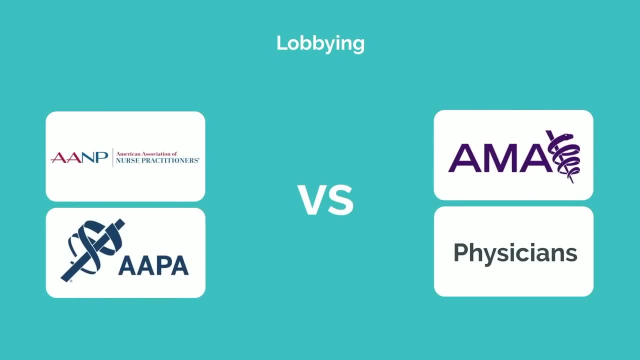 training and capabilities. Second, and more importantly, the AANP and AAPA are much more effective at lobbying compared to the AMA and physicians. It's easy to point to the insanely demanding schedules of physicians, but they're not the only ones who have to.